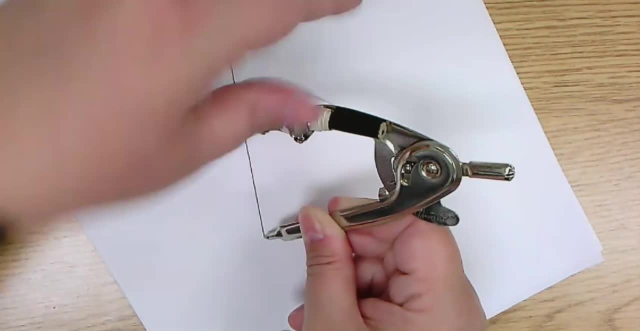 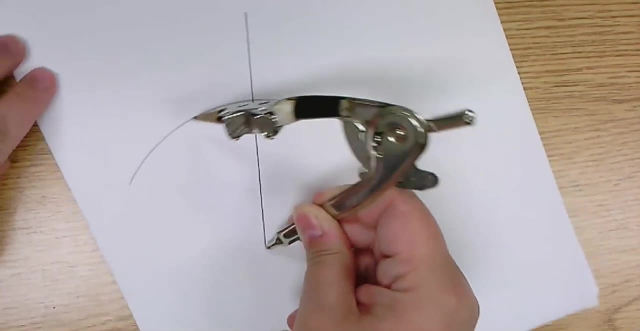 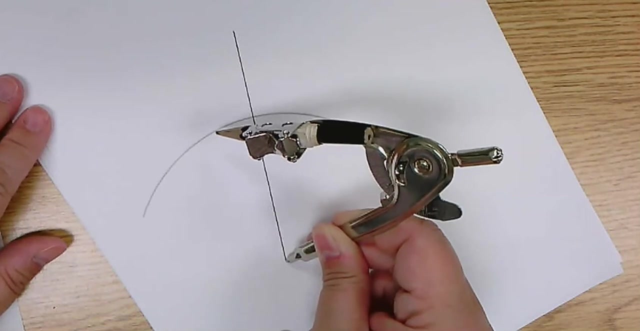 place, Not on this side, where the writing surface is not up top. Don't hold it any of those places. Hold it here. That'll help you with stability. Another thing is you notice I was turning the paper. that can help And then finally notice that you can see all of the compass because I don't have it. 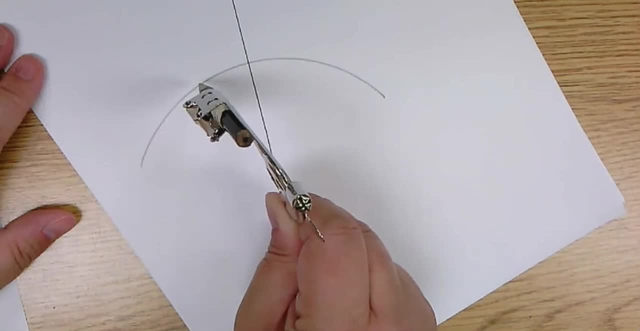 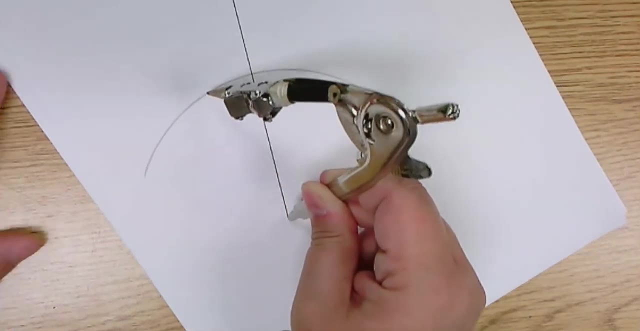 straight up and down. This would be straight up and down because the camera is above my paper, So you don't want to hold it straight up and down perpendicular to the paper. You want to hold it at an angle? Okay, and then you can draw your arc. Now, a lot of times we do constructions, the key. 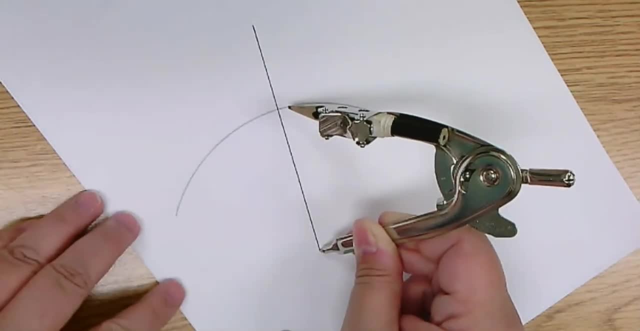 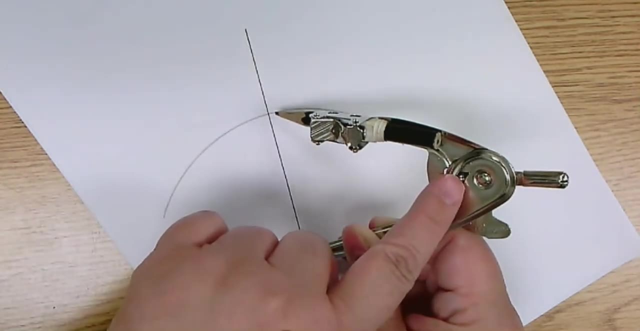 is that we're going to do one arc in a certain place and then we're going to do a matching arc exactly the same size. Now, if you're using this type of compass, it's important that it's able to stay put in terms of 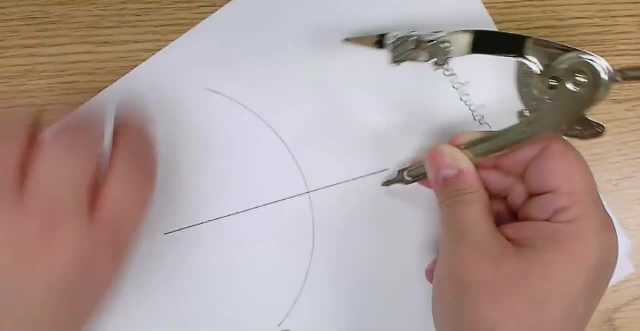 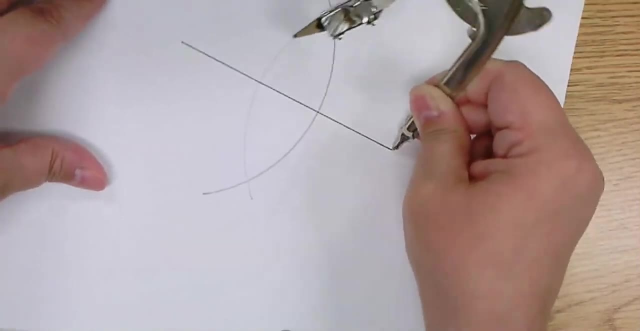 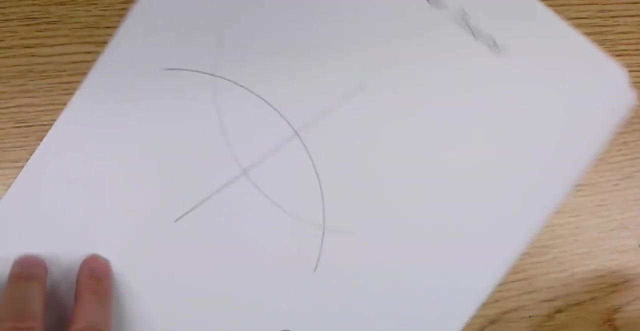 however much you open it, It stays open that much when you go to draw the same size arc somewhere else. So I'm going to the other end of this segment: same size arc. So I have two arcs that are exactly the same size. Okay, and they are basically this is: 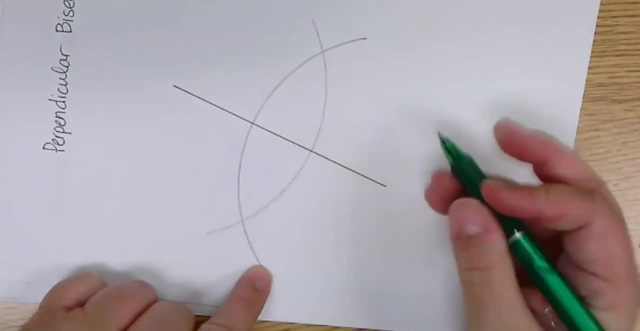 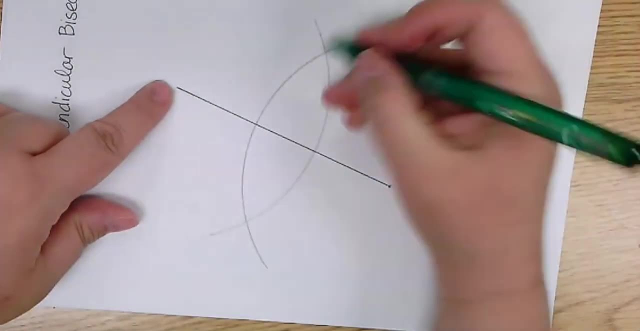 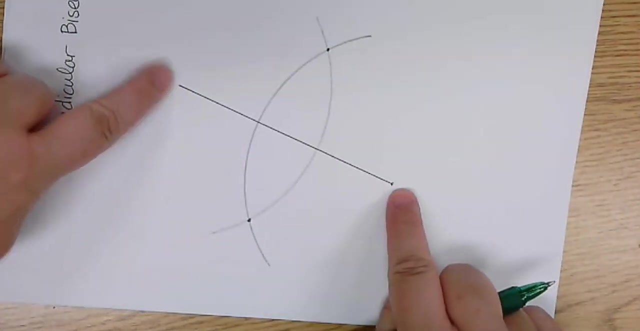 each arc is every point that is the same. This is the same distance away from this end point and every point on this arc is the same distance away from this end point. So these two points where my two arcs cross, where they intersect, those are points that are equidistant from both end points. And one of the things we learned about. 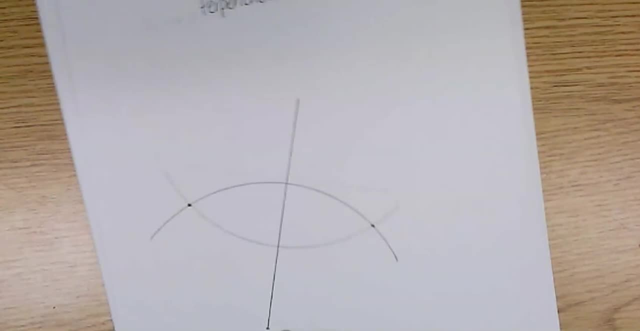 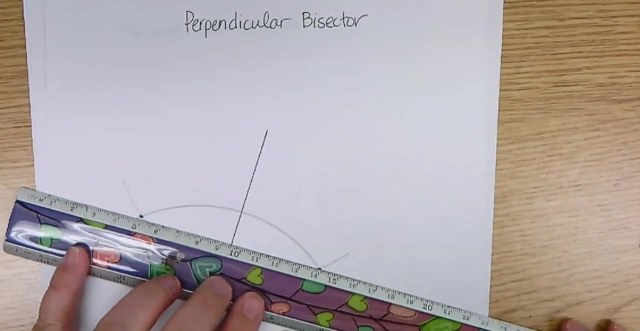 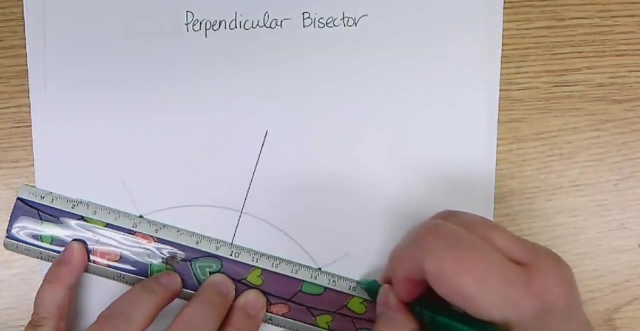 the perpendicular bisector very early in geometry is the perpendicular bisector theorem says: the perpendicular bisector is this sorry- is the set of all points that are equidistant From the end points of your segment. Okay, Now, usually when you're doing constructions, 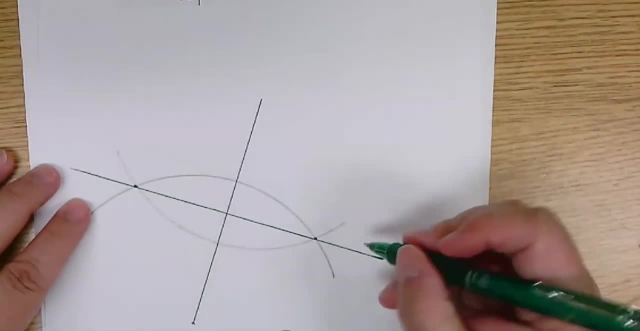 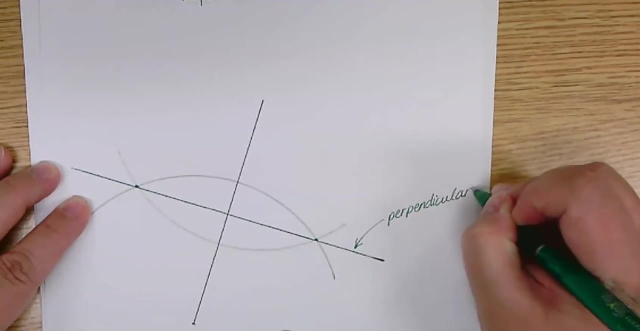 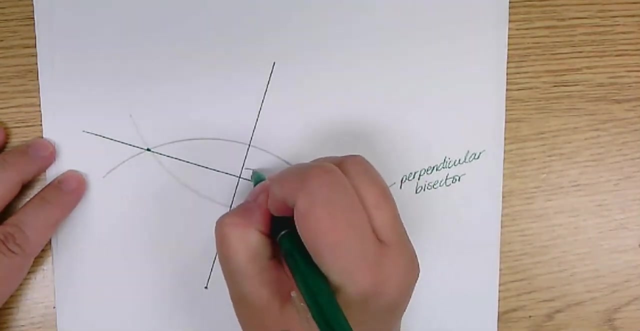 you don't do anything in ink. I went ahead and did this a little bit differently so you could see it. This is the perpendicular bisector. Sometimes, at the end of your construction, you are asked to mark it to show what it is. Perpendicular means draw a little right angle. 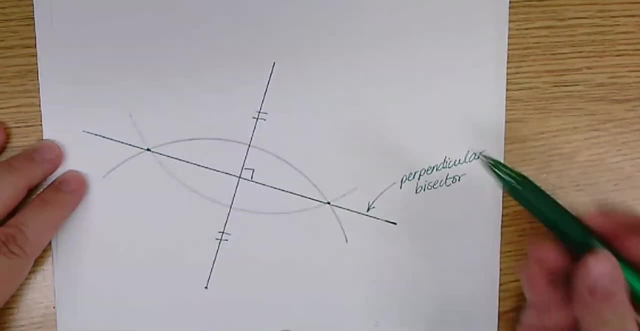 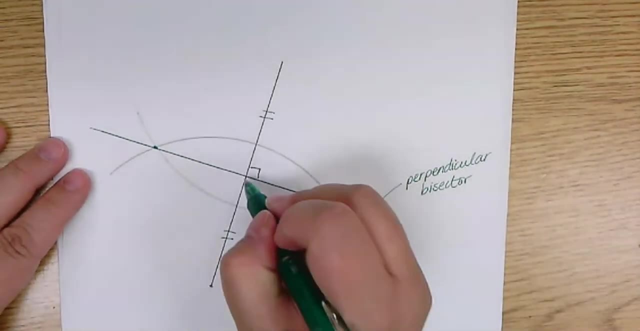 Bisector means draw congruence marks on either side that say this piece is the same, Same side as this piece or same size as this piece. Another thing that tells us is that this is the midpoint of my segment. So let me give this some letters here And I'm going to say I have created 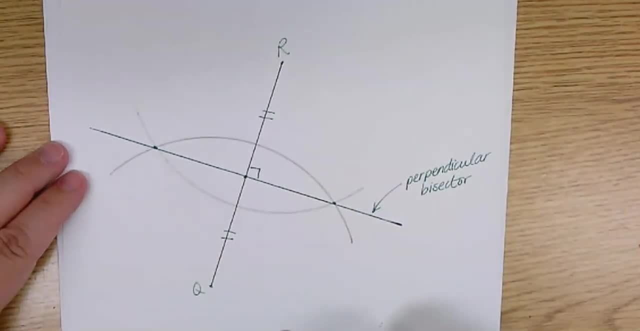 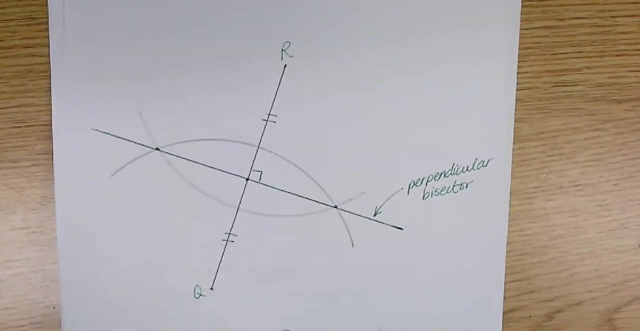 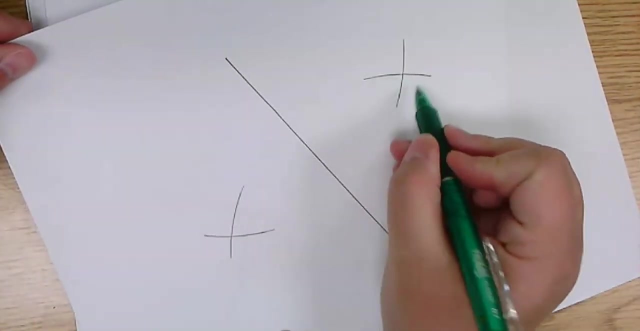 the perpendicular bisector of segment QR. Now, let me point out, if you look at videos online, sometimes instead of the arcs, like you see that I have done, sometimes, you'll see something that looks like this instead, where it's just two little pieces. 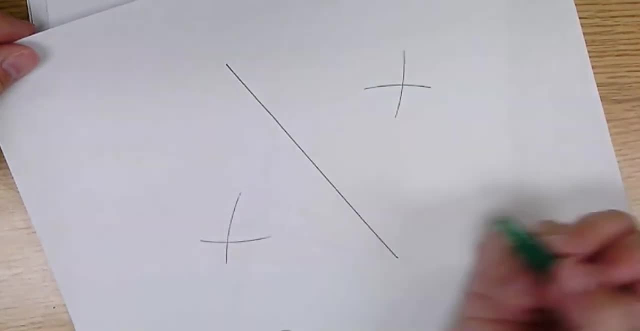 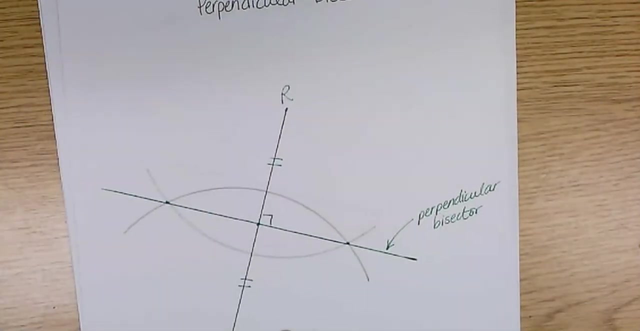 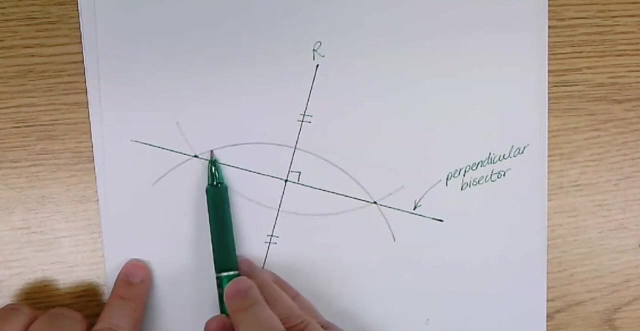 Of arc that are intersecting on either side. Okay, That is exactly done, exactly the same way. If it looks like this, don't look at mine and go: oh, she did it totally differently. It's really just that they didn't continue it from here to here. They did this part of the arc. 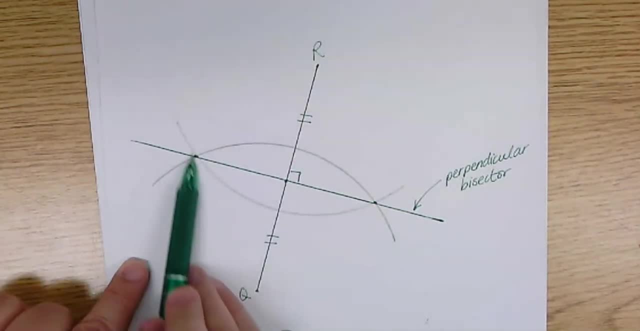 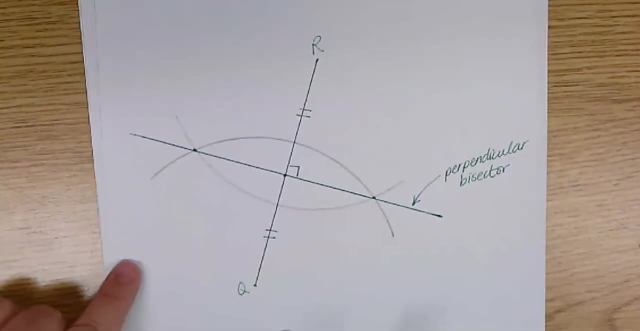 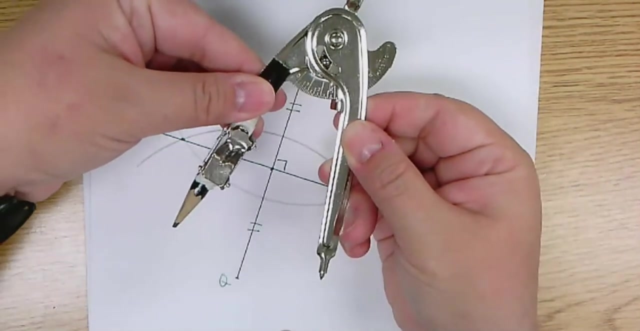 and then lifted the pencil and then did this part, did this part of the arc, lifted the pencil and did this part. I prefer to do the arc, the whole arc, And here's why, Because sometimes these guys wiggle, Sometimes it doesn't stay open exactly as far as you've opened it, which is the goal. 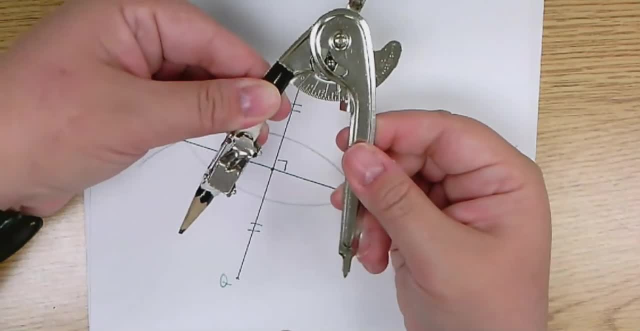 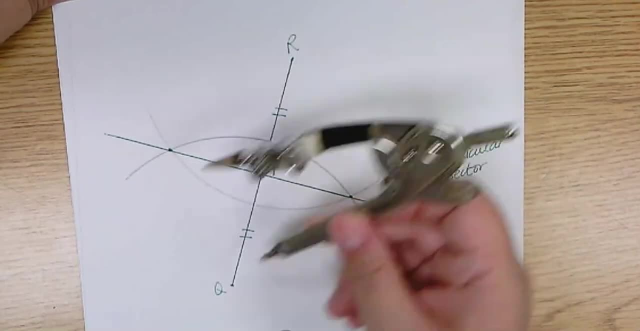 You want one that's tight enough that it stays put when you open at a certain distance. So one of the things we do when we're using these is we try to be careful not to make it wiggle, And to me every time I pick up my pencil and put it back down again. 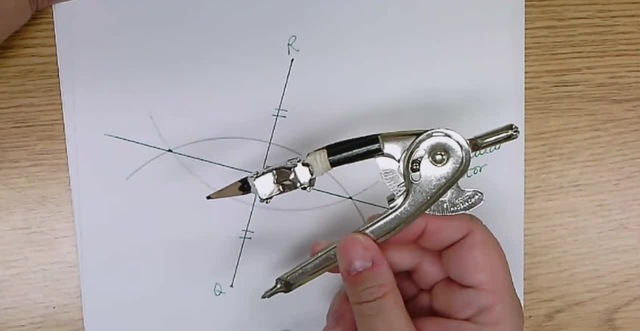 I've run the risk of changing just how far open it is. I run the risk of bumping it just a little bit, Nudging it open a little further or closed a little bit. So I would rather keep my pencil on the paper the whole way, draw the whole arc. 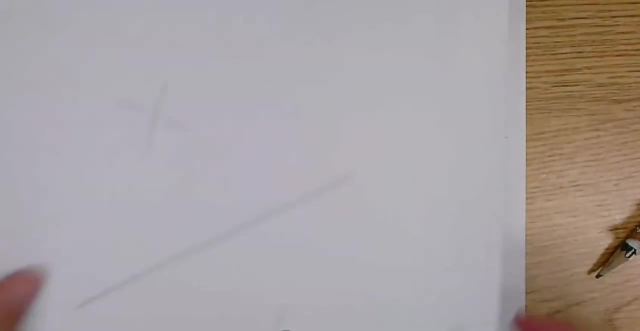 and then over here do the same thing. So don't think it's a big deal if it's this way In other pictures that you see, it's the same thing, And if you prefer to do it this way, that's absolutely fine. You will still, at the end, take the two points of intersection. 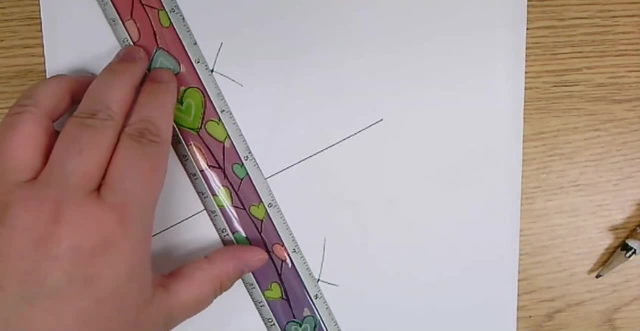 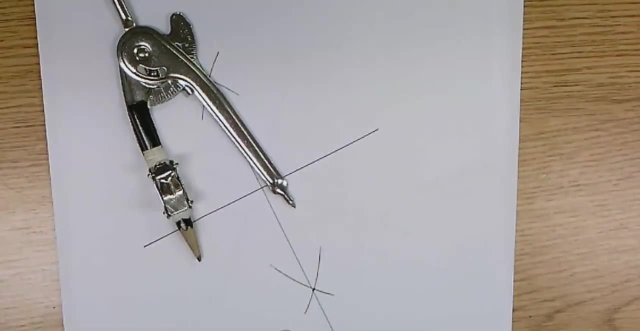 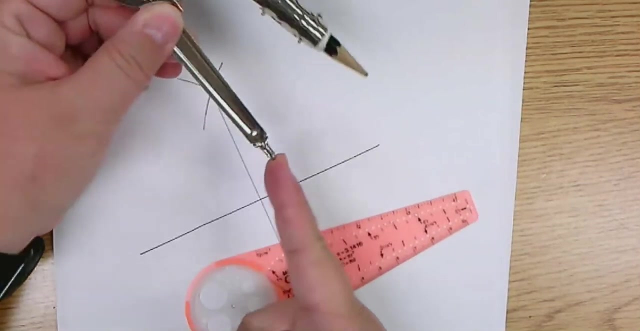 and connect them, And that will be your perpendicular bisector. Okay, so let's compare. Let's compare traditional compass to safety compass. Okay, first off, traditional compass has the non-riding tip it pivots on. It's very often metal, Sometimes it's plastic. That's the one you plant and then you 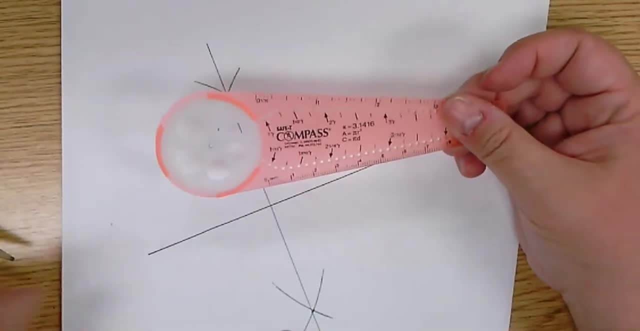 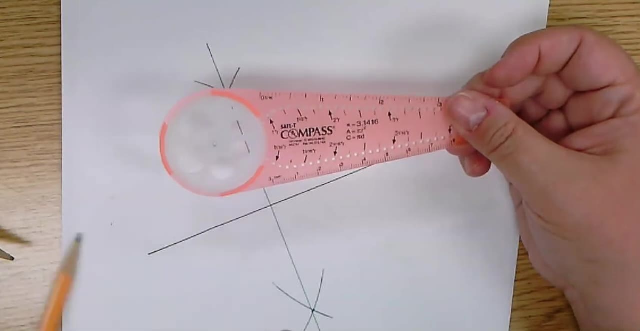 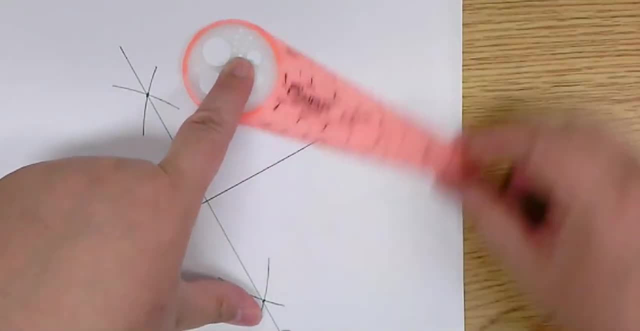 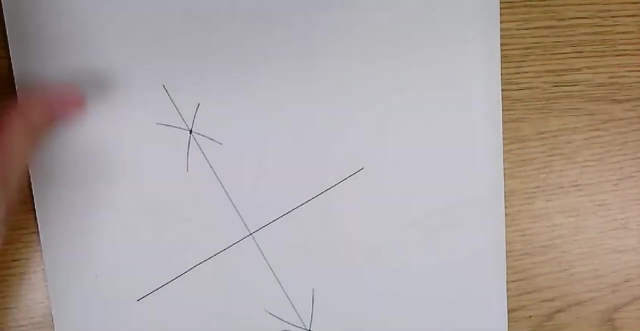 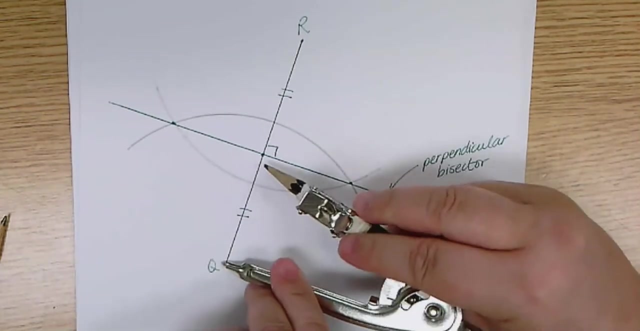 to plant this. hold the white circle down and then it spins freely. Okay, now another thing is. at the beginning of this particular construction, we said we're going to open the compass. I put my tip here. I said I'm going to open it so that it's more than halfway. 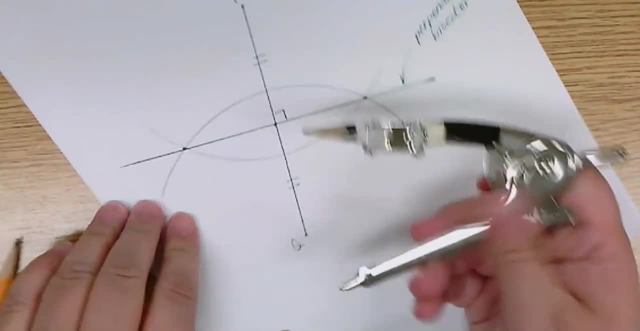 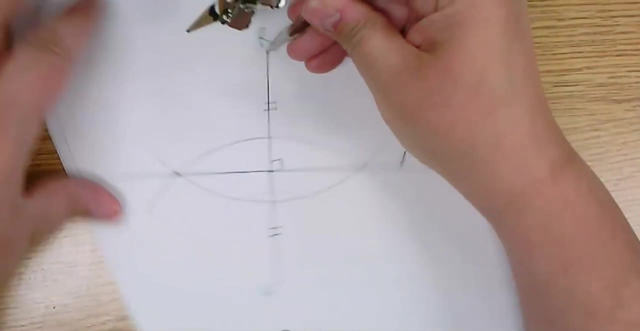 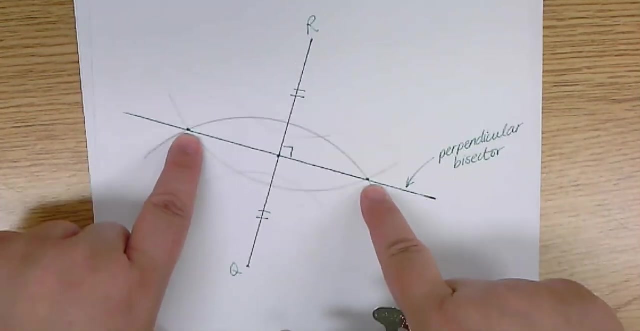 across. Let me point out, if I had not done that, if I had not opened it wide enough, that it was more than halfway across. what would happen is I would have a couple of arcs That don't meet. We want them to meet twice, so that's why it had to be more than halfway across. 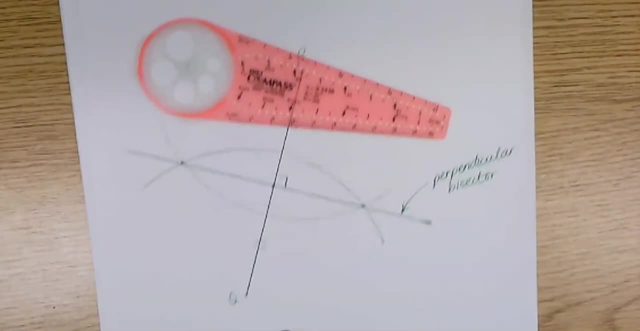 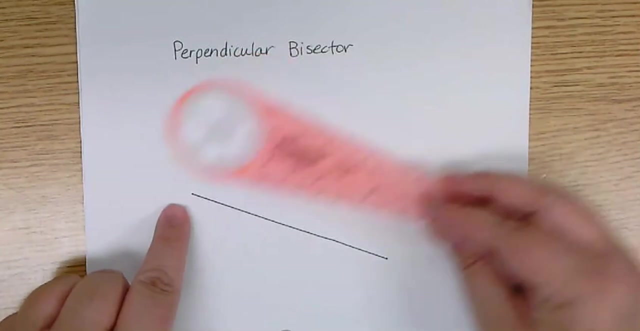 Okay, so what do we do here when we're told to open it a certain distance? Basically, that's about choosing a point, So let's go ahead and do the perpendicular bisector of this segment using our safety compass. I'm going to put my tip over one end point of the segment. That's like my. 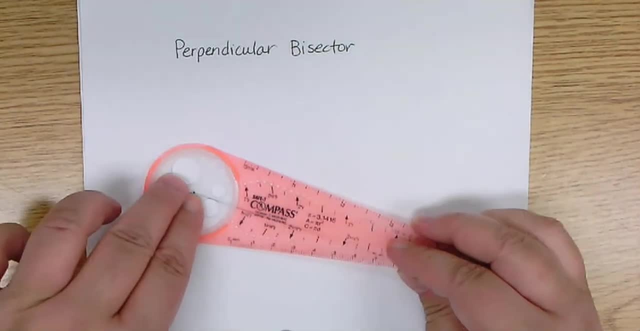 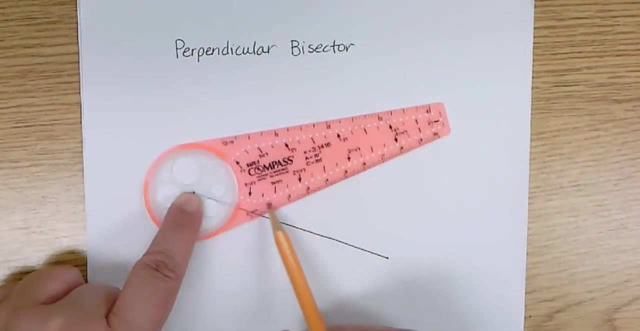 tip of the compass. I'm going to put my tip over one end point of the segment. That's like my tip of the compass, That's the center, And then, instead of saying open it a certain distance, basically you are choosing one of these dots to put your pencil in. You're choosing a point to put your pencil in that. 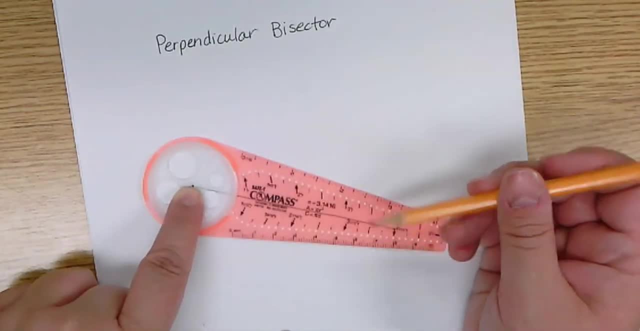 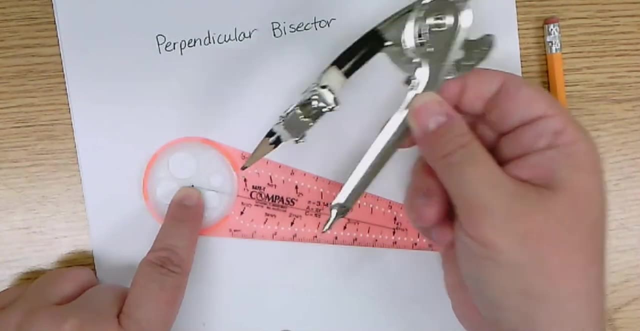 is more than halfway across. Now, the next thing that can be a challenge with this: if I'm using a traditional compass and I want it to do two arcs that are the same size, I just keep it open, the same distance, and I go from one place to another with the arc, the same distance, the two sides, the 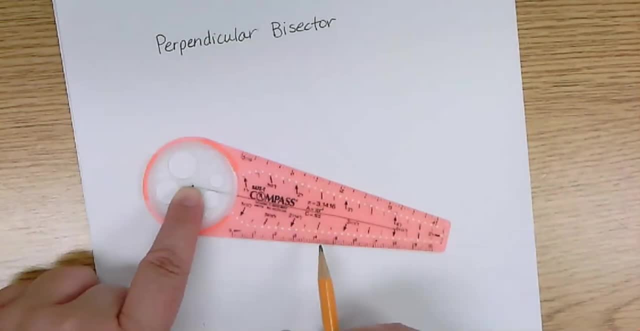 same distance apart Here, if you want to do two arcs- the same distance, which we very often do, that means remembering exactly which hole you put your pencil into, And I'm telling you that's harder than you think at first. Okay, so I end up doing with these. this is, to me, the only drawback of these. I end up doing. 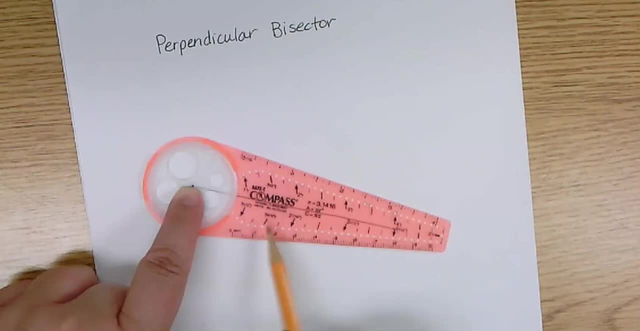 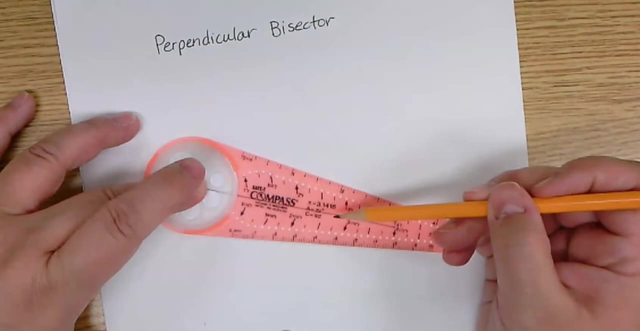 a lot of double checking- Wait a minute, which hole did I use again? And I go back and I check the last arc I drew. So if I want to draw an arc that has a radius that is more than half the length of the segment, I'm going to use this point. 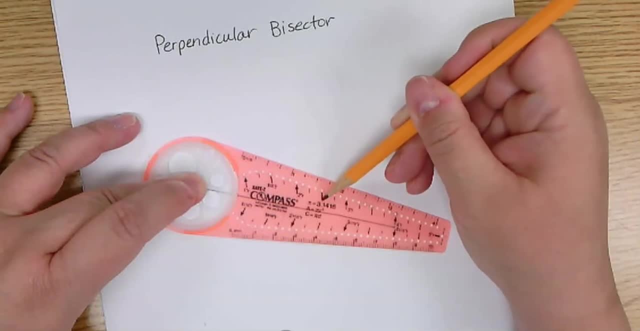 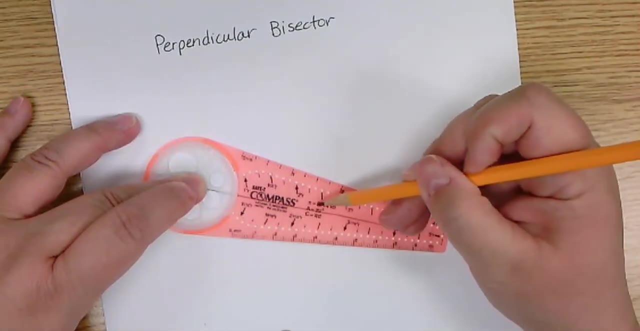 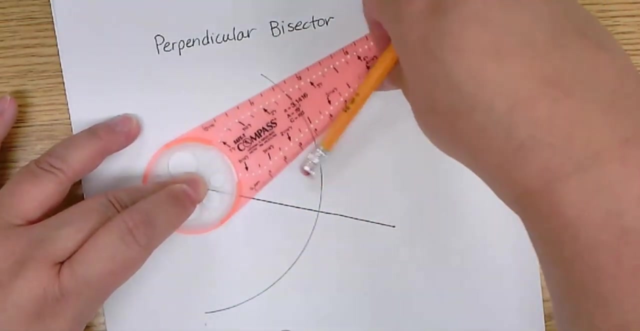 Here I like to choose dots that have some sort of identifying mark beside them, So I'm going to use that long, the dot right by the long mark here above the 3.14.. Okay, and I'm going to do that arc And then I'm going to move the pivot point, which is like the compass tip, to the other. 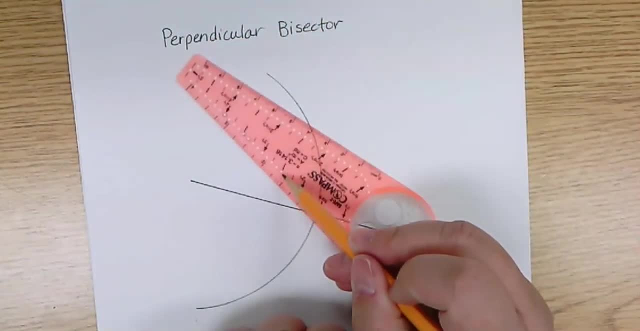 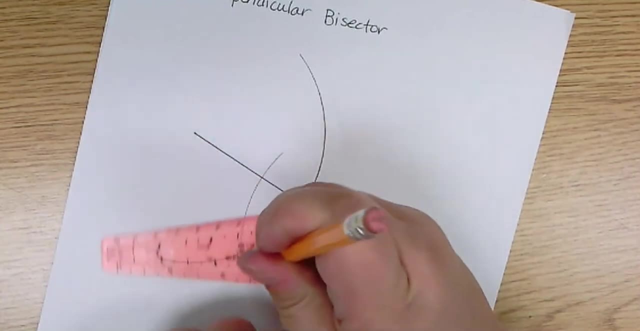 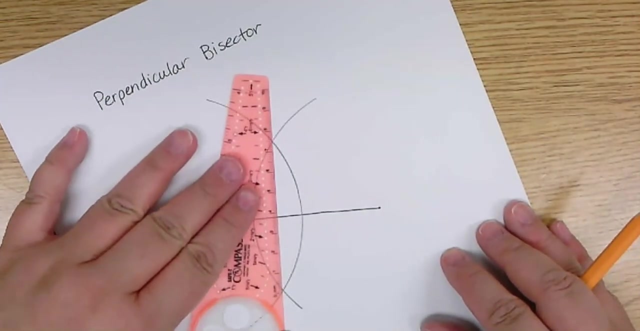 end of the segment And I have to use that same exact hole. I have to be able to go back to that hole- And it's even more challenging when it's upside down, because that was on the top on the other side- And do that same size arc from over here And then again I will connect the two points of. 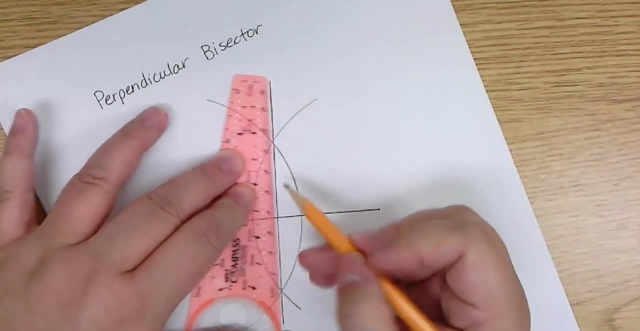 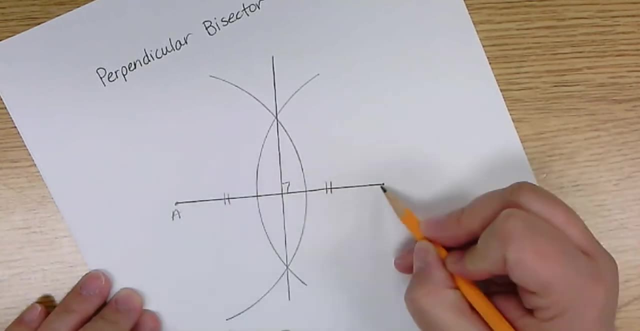 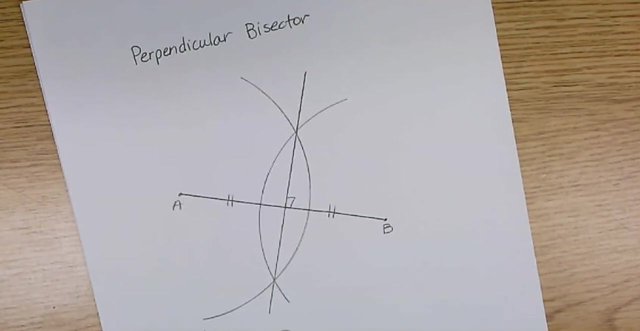 intersection And that's my perpendicular bisector. It's perpendicular to the segment And it cuts it into two congruent pieces, The perpendicular bisector of AB. Now, one thing I want to point out to you is that if you're going to draw an arc that has a radius that is more than half the length, 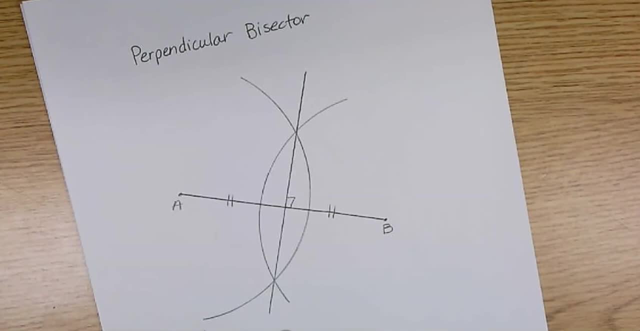 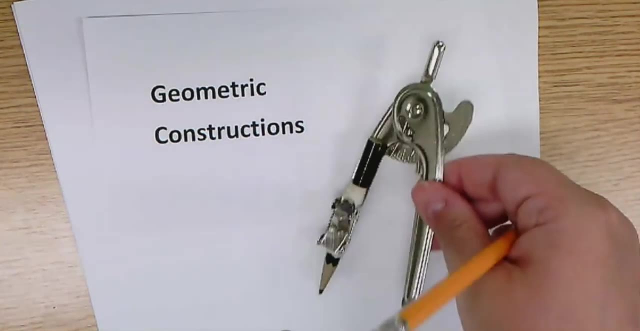 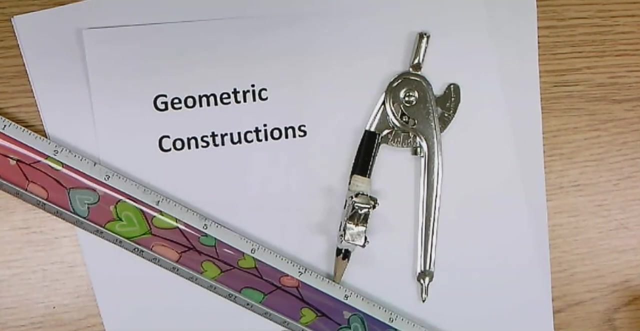 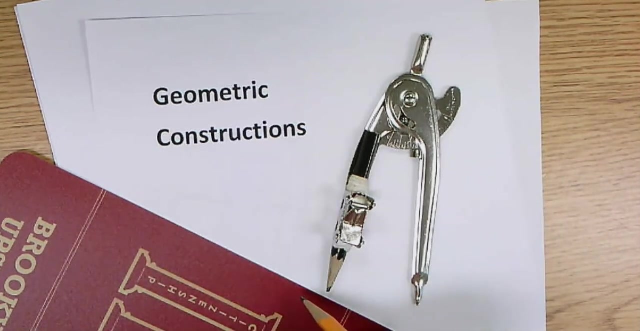 of what our reversedır friends are going to be, and I will show you in the basic examples that we had them in num. it's going to be somewhatᅠ gluon. That could be my straight edge, all right. So a compass and something to help you draw a straight line. 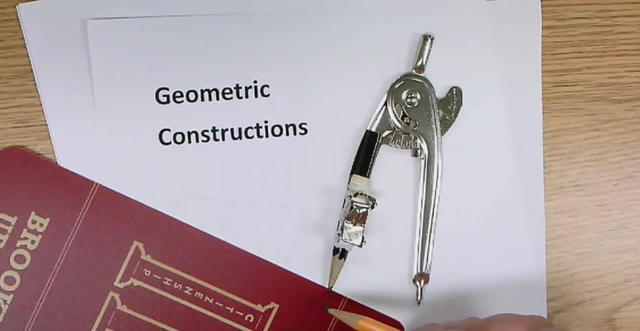 There's no measuring involved. You will never measure any degrees, any inches, any centimeters, anything like that, when you're doing constructions. okay, So we just need something to draw the arcs- that's the compass- and something to connect points by a straight line. 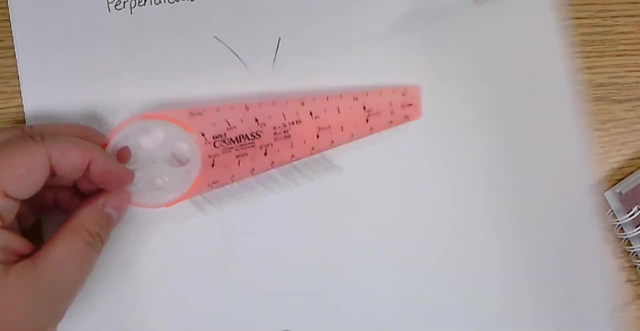 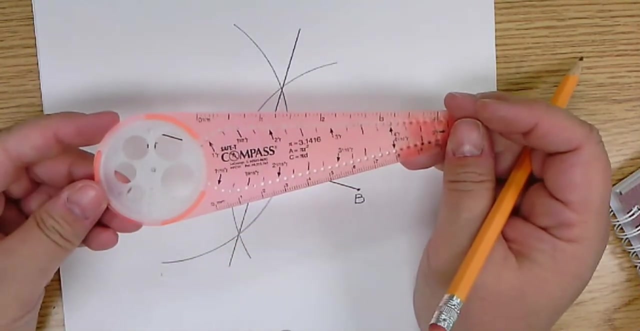 That's the beauty of this one is it's both in one. You notice that when I went to connect these, I already just used the edge here, So this does the arcs and it's the straight edge as well. So that's the nice thing about the safety compass. 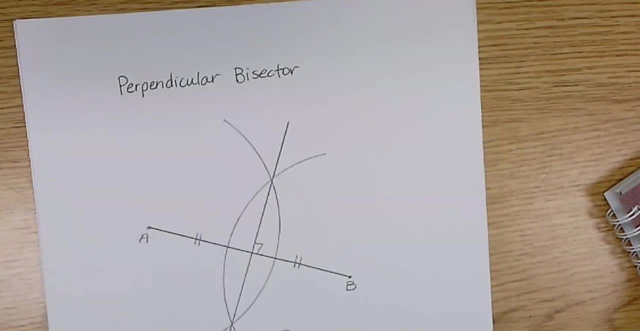 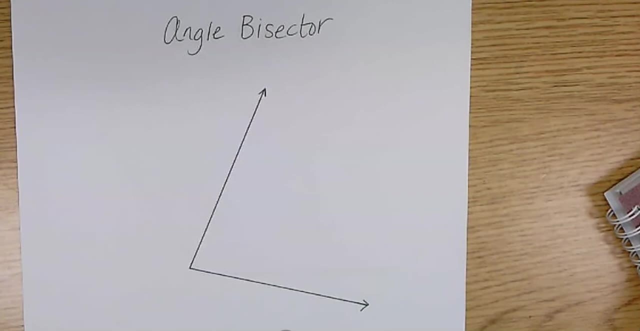 Okay, I want to show you one more basic construction, and that's the construction of the angle bisector. All right, let's do it with a traditional compass first. The first step is, I put my compass tip on the vertex of the angle bisector. 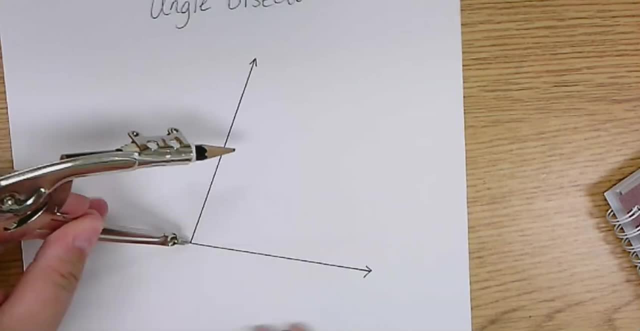 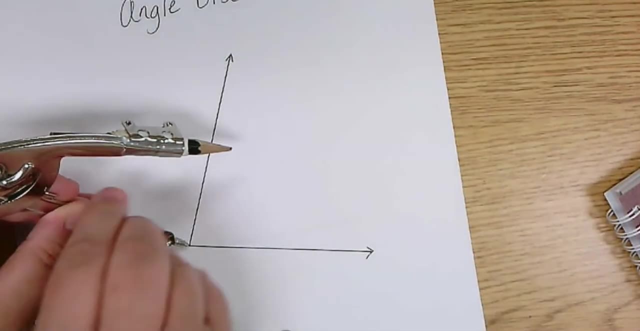 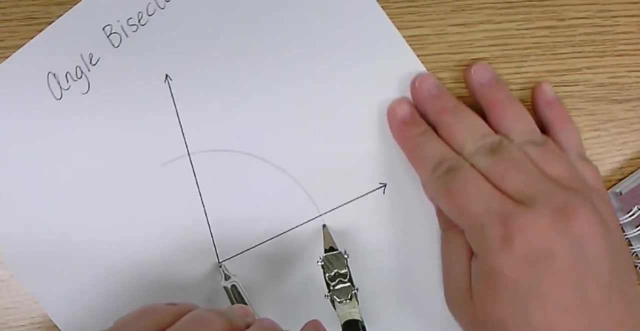 And I open it any distance I want, as long as it's not beyond the edges of where I've drawn my angle. Because what has to happen here is I have to draw an arc of any size that crosses both sides of the angle. It doesn't matter what size. 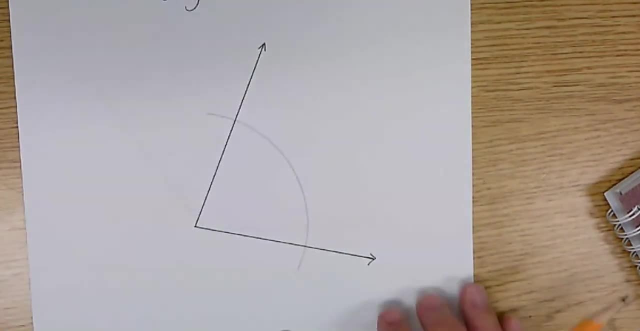 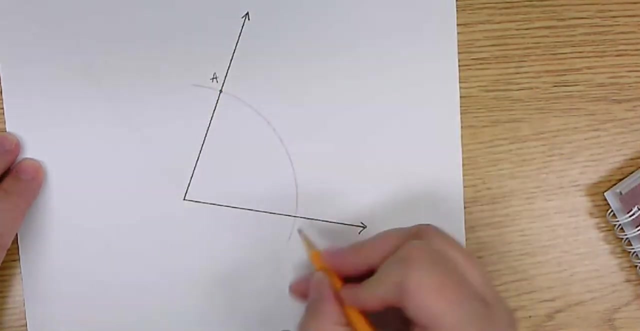 it just has to cross both sides of the angle. Now, the reason we did that is because that gives us two points. Here's one point, Let's call that A, And then another point, we'll call it B. What we know about those two points is that they are: 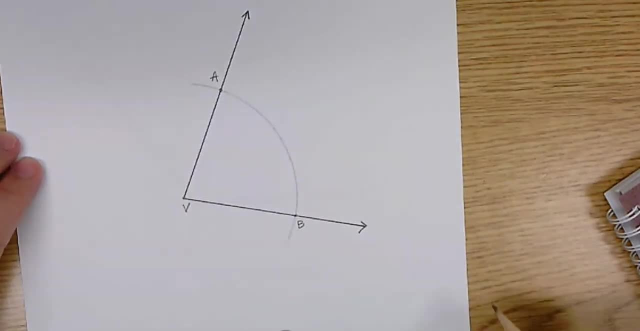 equidistant from the vertex, which I'll call V. The distance from V to A is the same as V to B. So now what I'm going to do is I'm going to draw two more arcs, one with the point on A and one with the point on B. 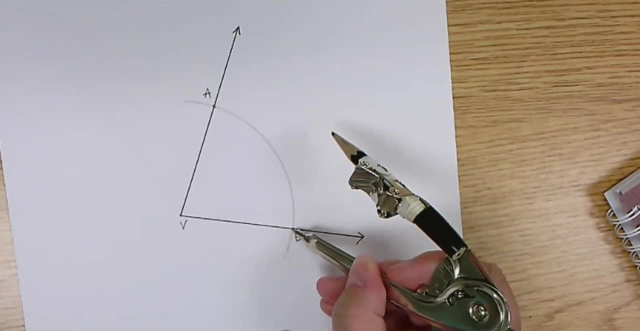 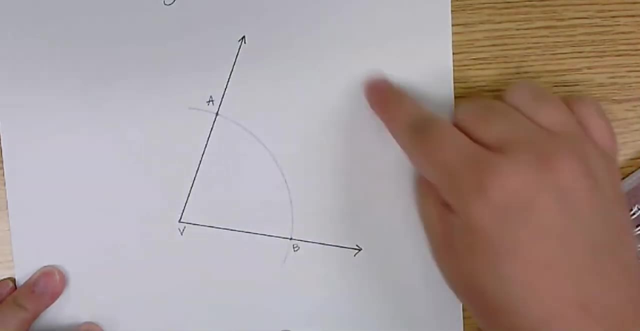 These next two arcs have to be matching in size And in terms of where. they just have to be somewhere out here in the interior of the angle. I usually like to draw them somewhere around here. The goal here is to make two arcs the same size. 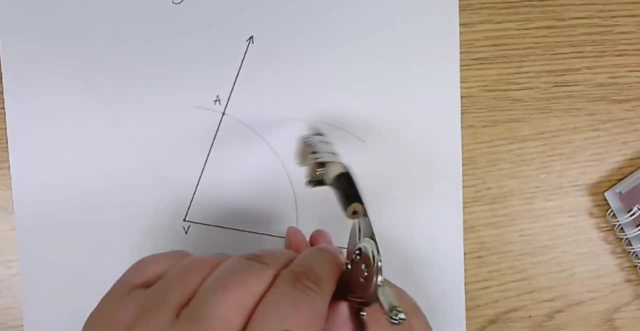 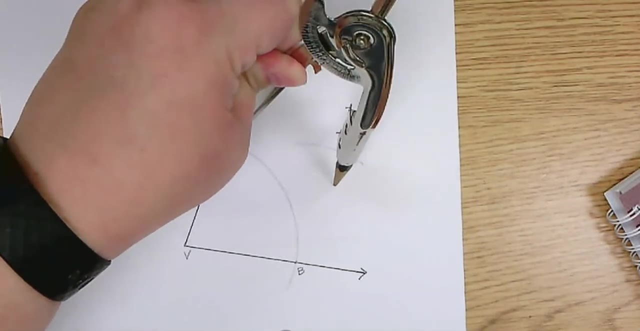 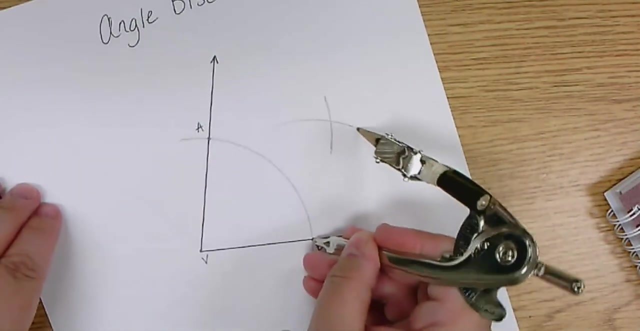 and put them someplace where they will cross. Remember to make the arcs the same size. you've got to make sure your compass does not change when it switches from going over here to over here here or vice versa. So I have accomplished my goal, which is the two arcs crossed, If your two. 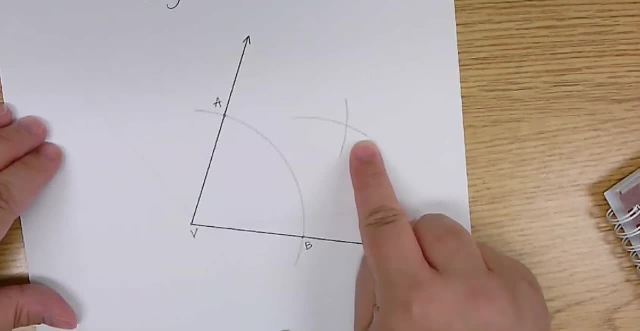 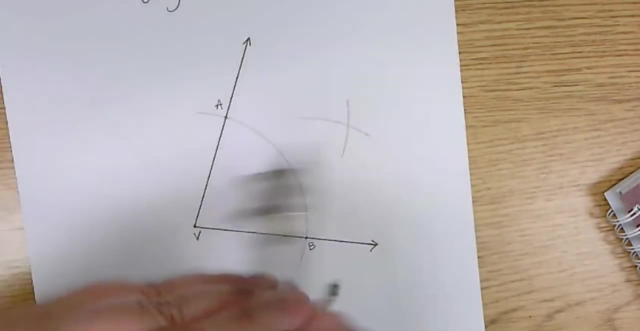 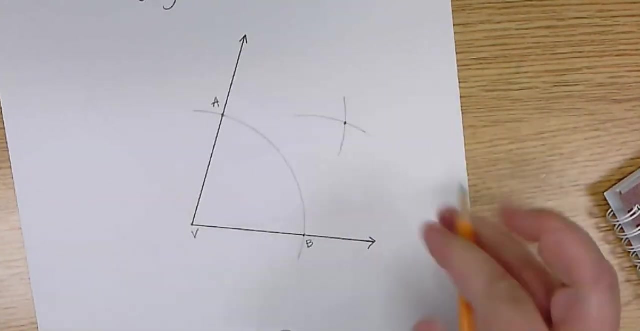 arcs didn't cross. try doing a different size arc or try drawing it in a different place, but make sure that they're the same size from each point, that whatever you do from over here matches what you do from over here. And the last step is I take that point of intersection and I connect it back. 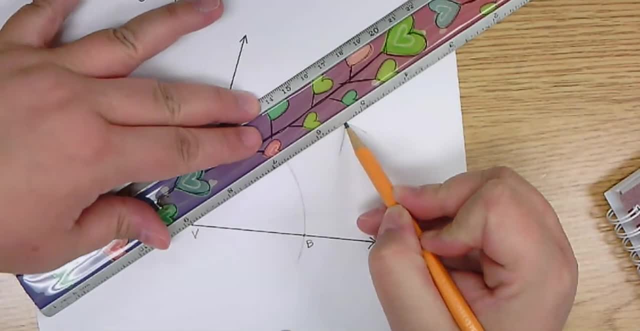 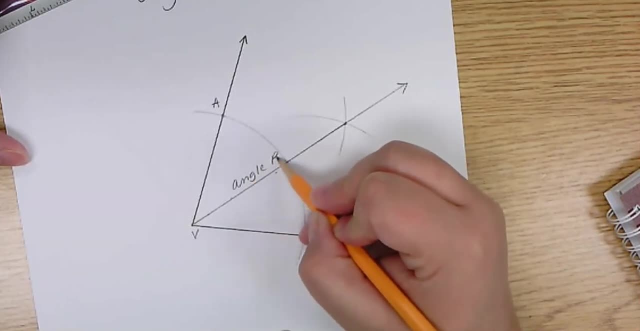 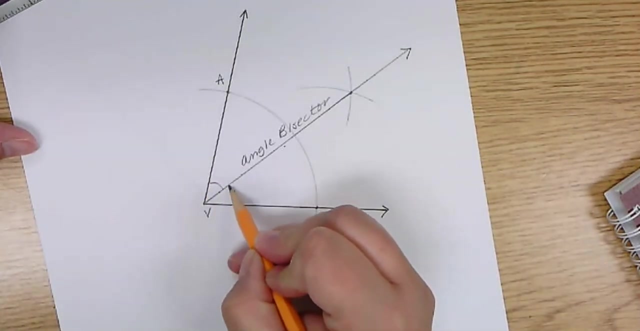 to the vertex of the angle and that's my angle bisector. And there it is. That is the angle bisector. And how do we mark it? Not usually by writing the word angle bisector, We mark it by showing congruent symbols on either side, congruent little arcs. So I have created the angle bisector. 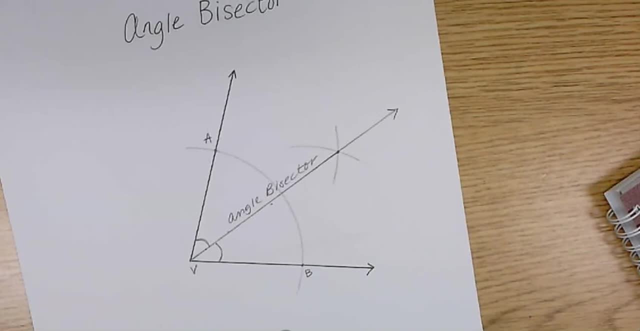 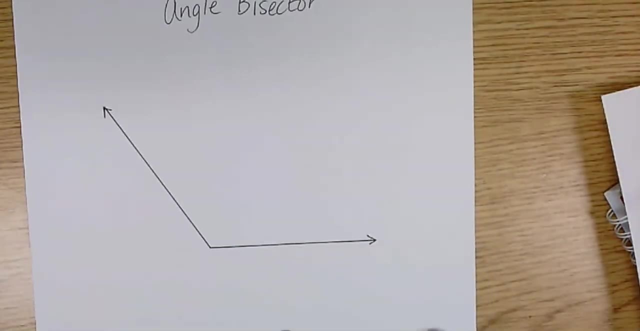 of angle A, V, B. Let's do those exact same steps, but this time with the same angle, bisector. So I'm going to take my safety compass a little bit bigger angle- Remember the first step- and I'm going to put 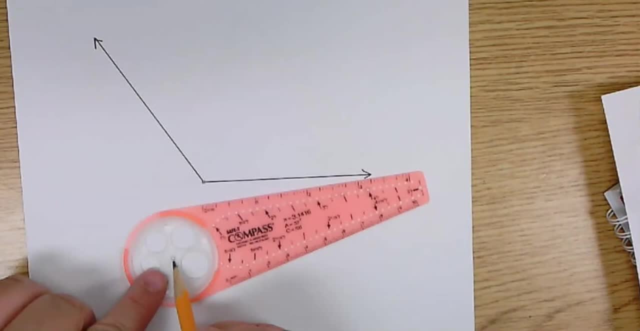 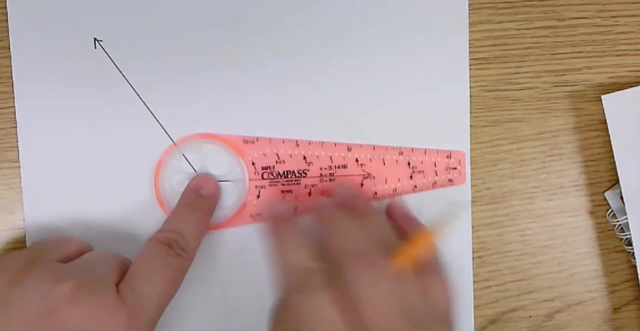 the center here of my safety compass. I'm going to put it over the vertex of the angle so that I can see it through that middle hole right there. I'm going to draw an arc. I'm going to pick any point I want to, as long as my arc will cross both sides of the angle. So I'm going to pick a point I can. 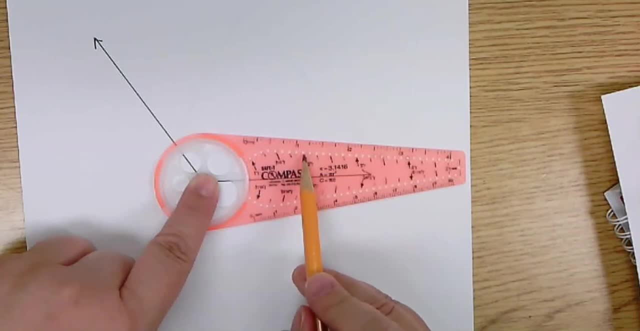 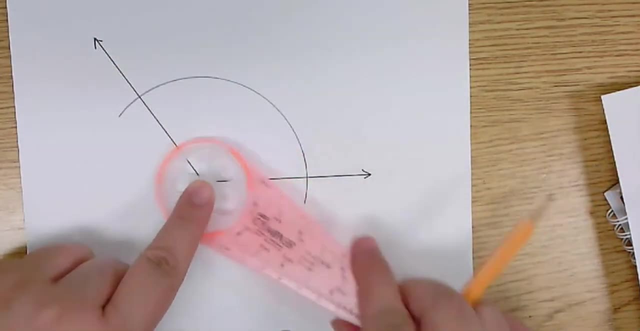 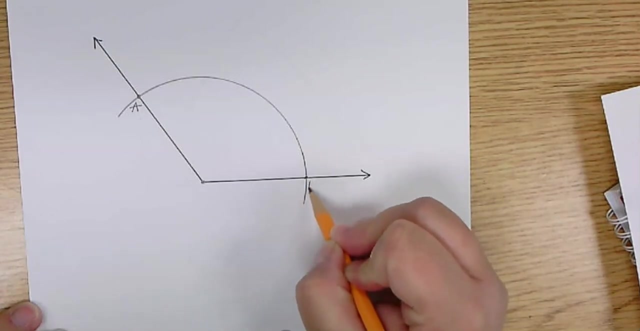 remember, I'm going to pick this point that has an arrow pointing to it right up here, although it really doesn't matter. I'm only doing one arc this size. Okay, now, that gave me two points, One point on one side and another point on the other side, And again we'll go ahead and call this V. 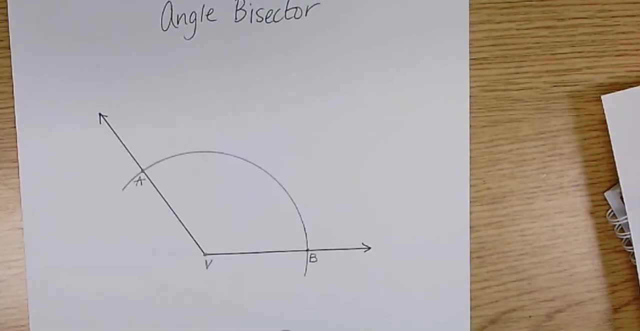 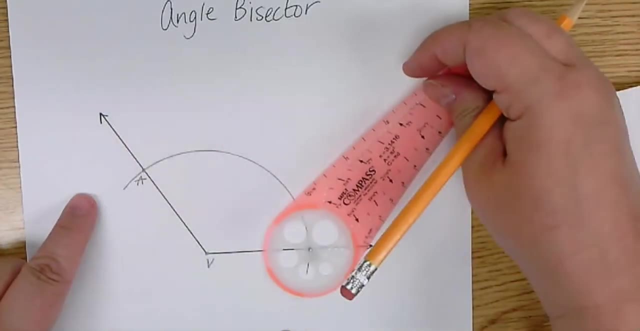 for my vertex. So now I'm going to draw two more arcs, one with the center of my compass on A and one with the center of my compass on B, And they have to be the same size and they will meet somewhere out here. 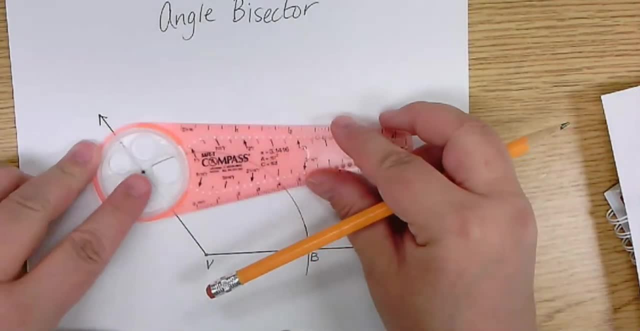 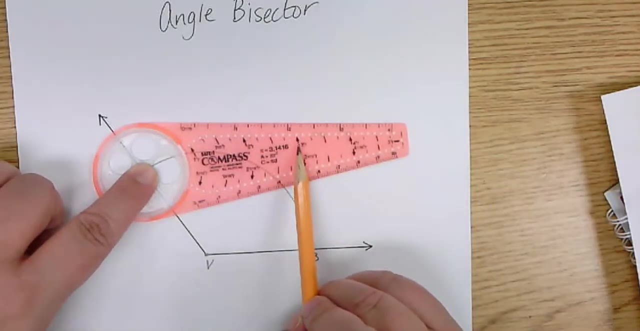 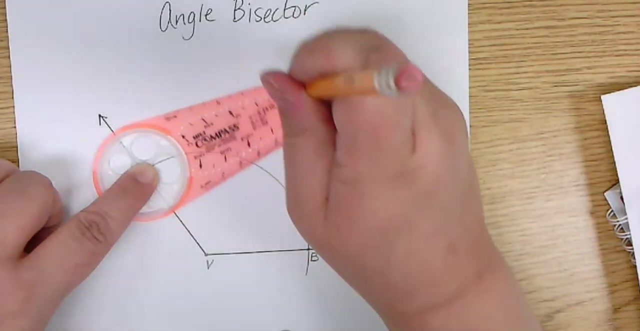 So, again, in terms of making them the same size, it helps, if I try to pick a hole, that I'll be able to remember which hole I used. I'm going to use this one here that has an arrow and has a three right next to it. three inches and an arrow, Okay, and I have to remember that's the point I used. 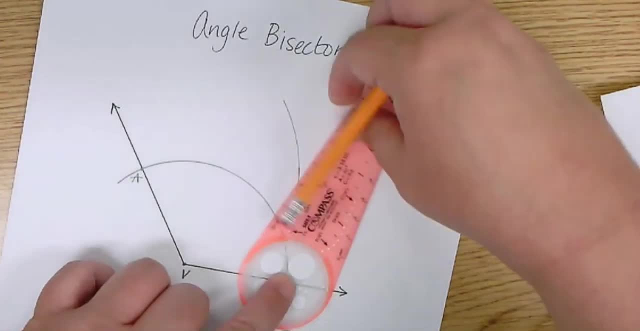 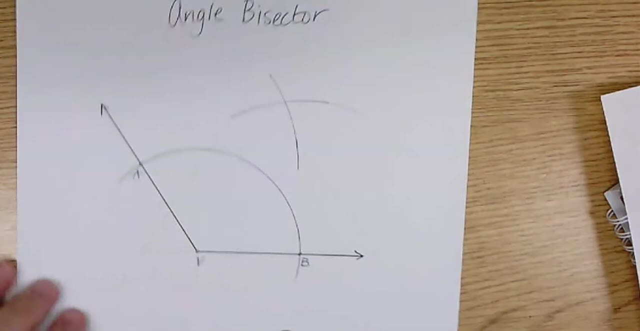 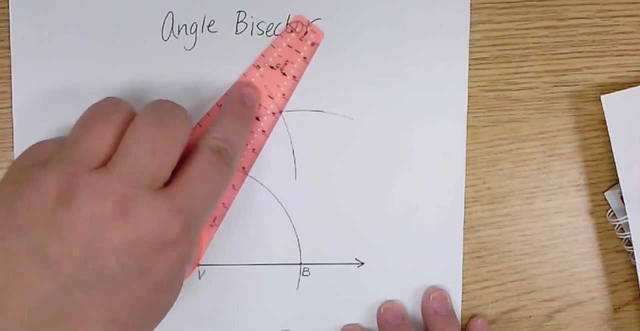 and come over here, put B right up underneath that hole and use that same point. My pencil has to go back in the same hole that it was in, And now I will take this point of intersection and connect it to V, And that's my angle bisector. 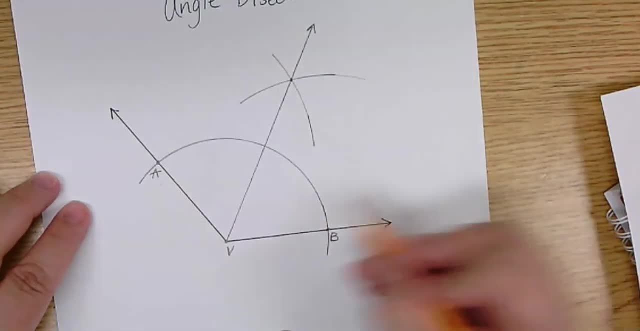 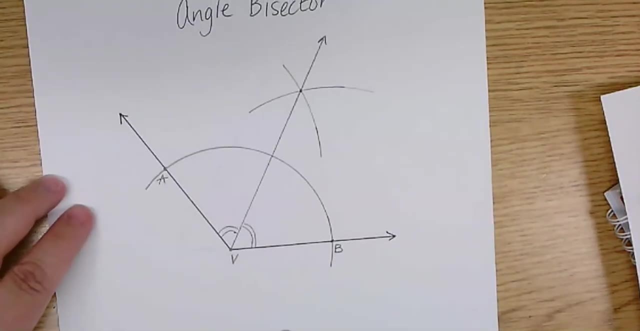 So this is the angle bisector of angle A, V, B, which means this angle over here is the same size as this angle over here. All right, last thing I want to show you on this video. this video is going to be: 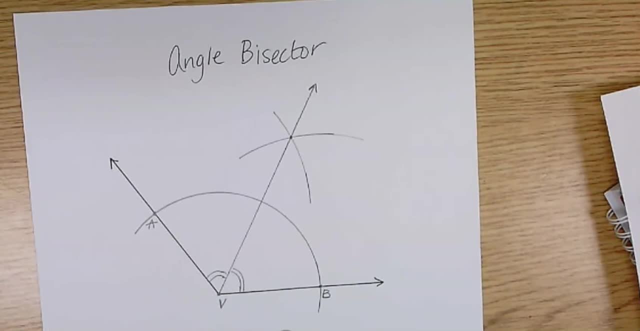 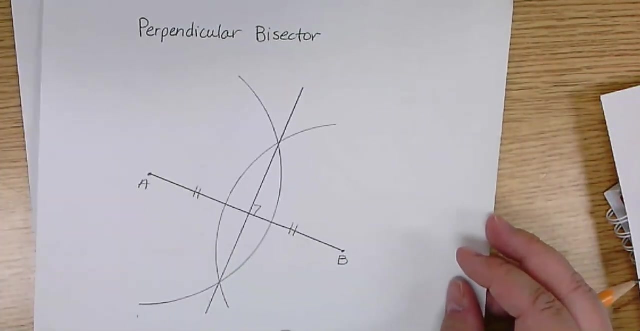 the perpendicular bisector and the angle bisector. Sometimes you are asked to do those things of triangles. So what I want to point out to you is, if you are asked to do the perpendicular bisector on a triangle, usually what you're going to do is you're going to do the perpendicular bisector. 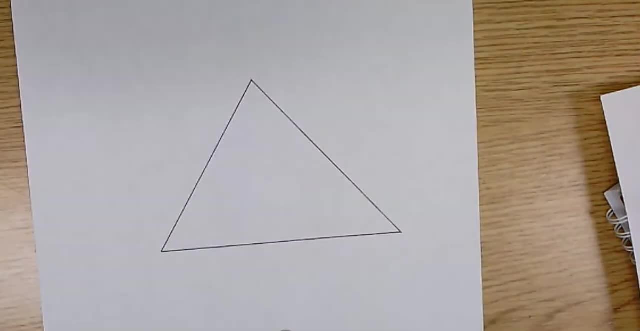 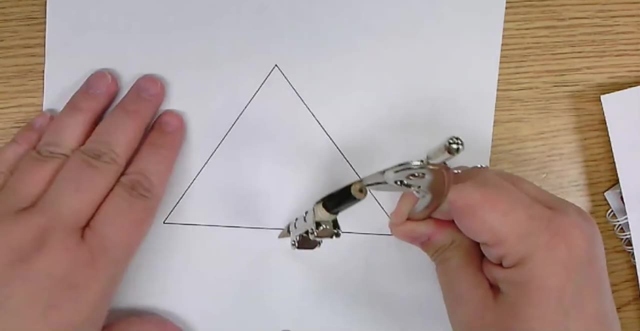 of each of the three sides. So the way that would look, and I'm just going to go through this real quick. but you do the whole process for perpendicular bisector, Basically ignoring every other side other than the one you're looking at right now. 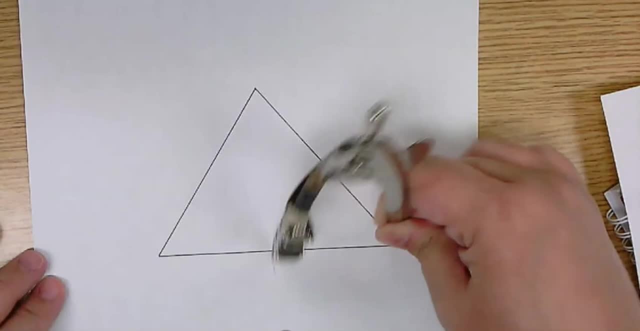 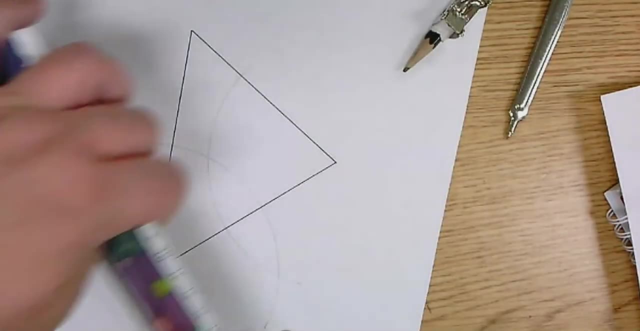 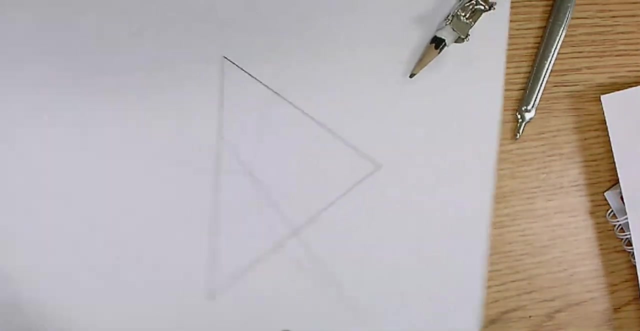 So I just do it for this segment, And then I go to a different segment and I ignore the rest of the triangle, And so now I'm just going to do it for this segment. All right, I'm going to use the safety compass this time. 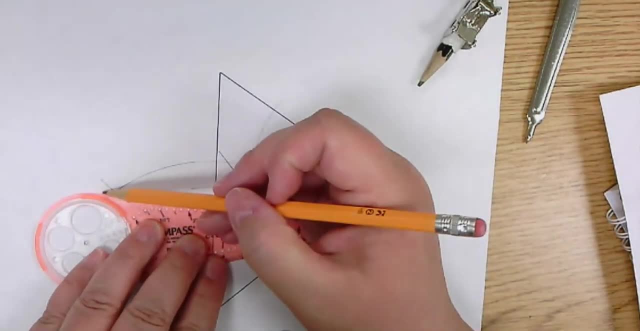 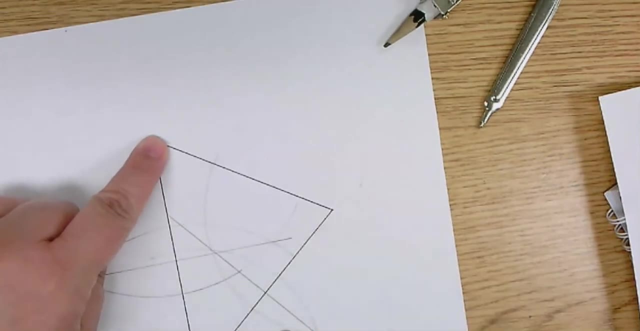 It looks a little messy. What happens is you've got it going on three times. This is going to be a little messy, You've got stuff overlapping And then, finally, we haven't done it to this side, So you just have to look at it very individually. 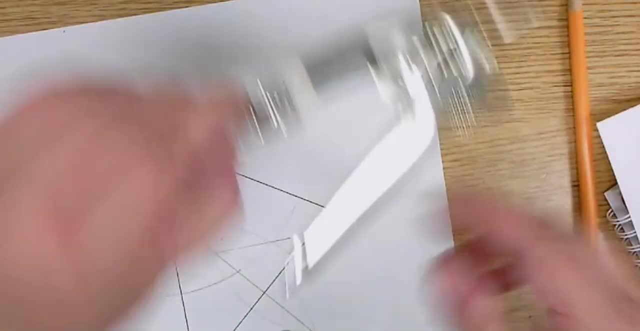 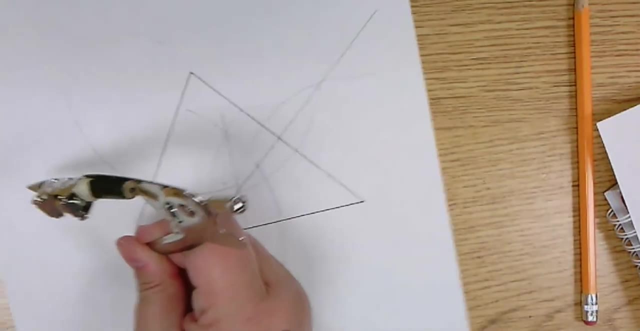 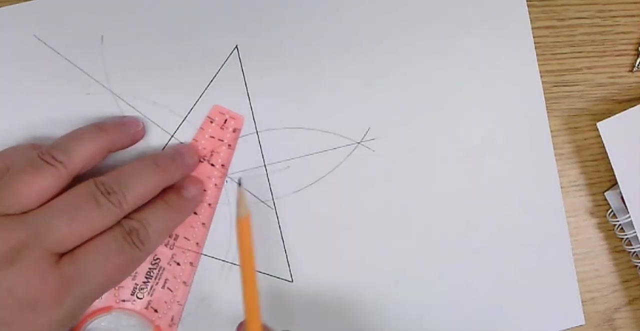 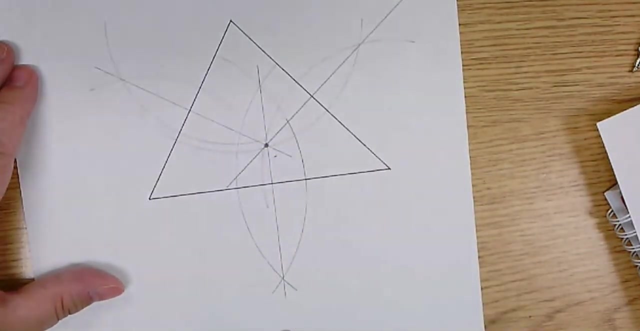 One side of the triangle, One side of the triangle at a time, And do it for each side of the triangle, And I did this really fast. but if you do it carefully and correctly, what you'll notice is all three of these perpendicular bisectors of the sides will meet at a single point. 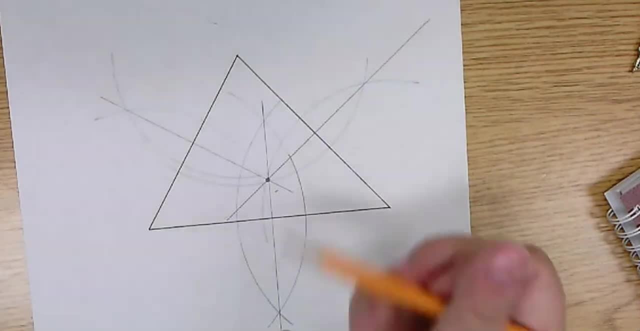 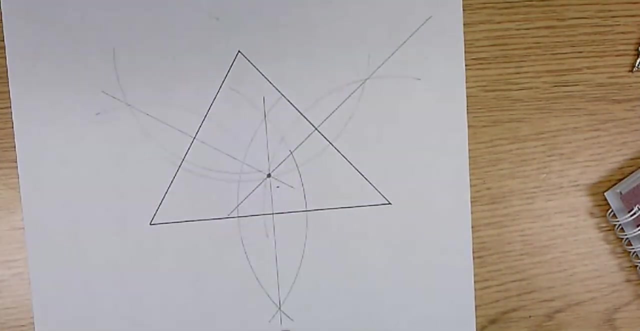 And that's generally when you are asked to do this Is when you're exploring the properties of that point- has a special name. It's called a triangle center. These lines are called concurrent because they all meet at one point And that particular point is called the circumcenter. 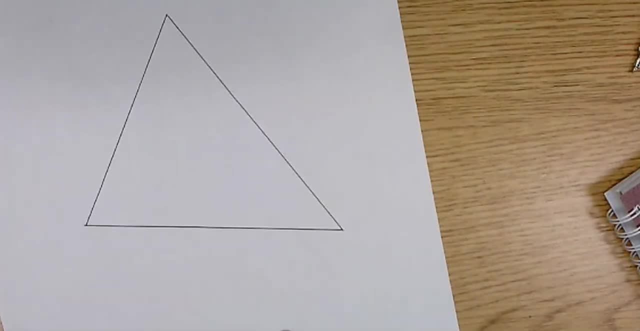 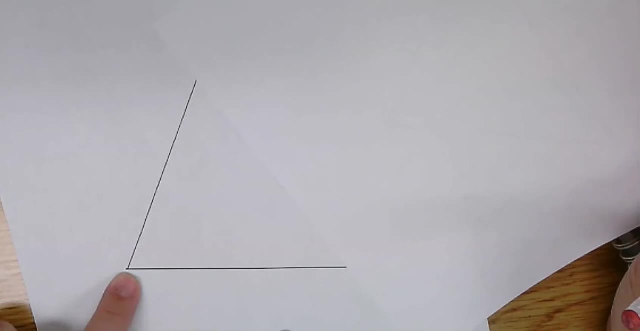 You could do the same thing with the angle bisectors: Just look at one angle at a time. So if I'm picking one angle at a time that's like let's say it's this one, It's like I don't think of it as a triangle. 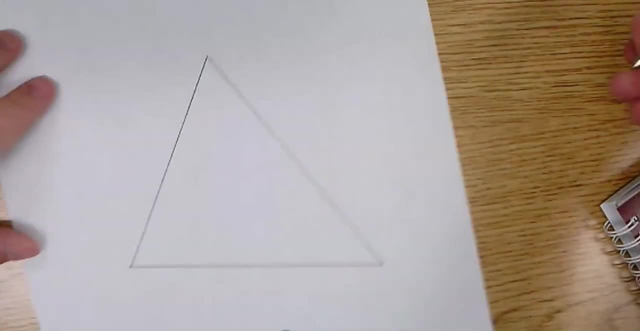 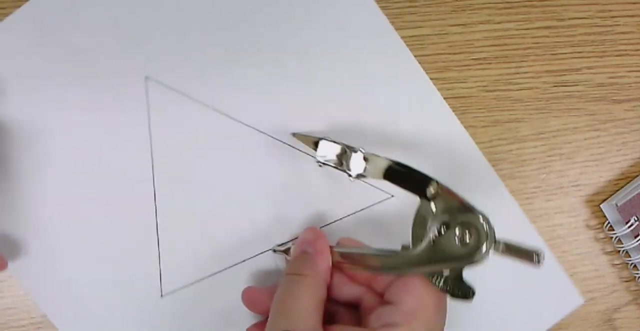 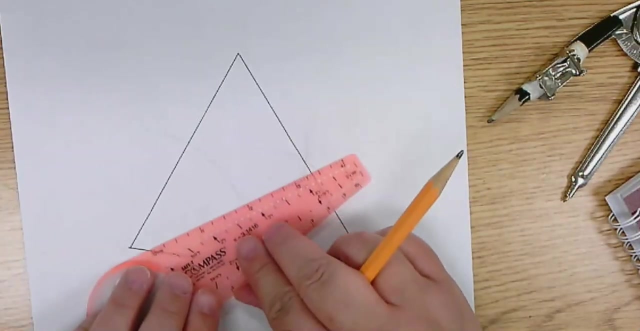 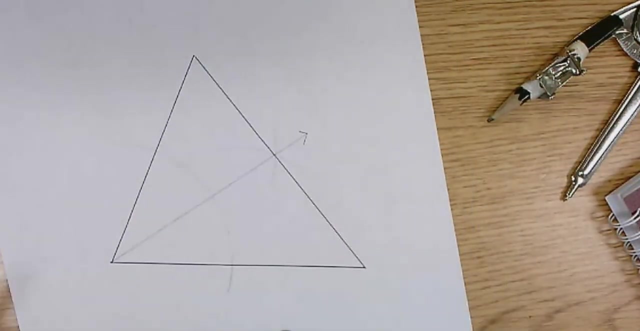 I just think of it as an angle. So I'm going to draw an arc that crosses both sides of my angle And then two new arcs from those points And I connect that intersection back to the vertex And I keep doing that one angle at a time. 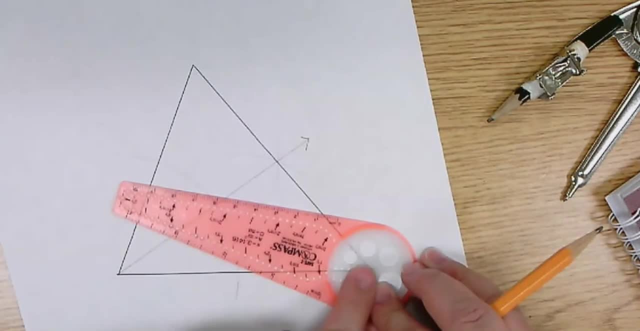 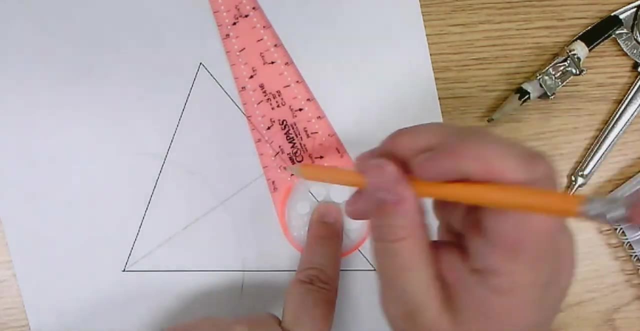 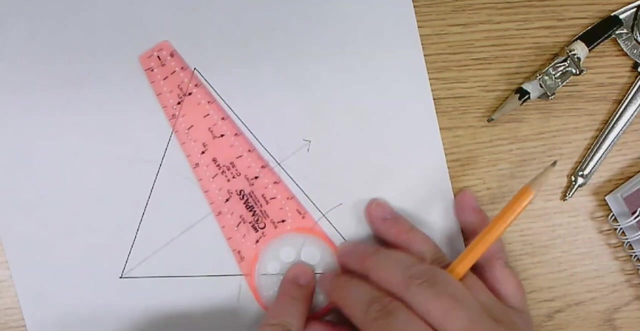 So, like I could do it over here, Draw an arc that crosses both sides And move to this point And draw an arc And move to this point And draw the same size arc I just drew, So I have to use the same hole.